general intelligence, this is not ASI, this is not AGI, but it will work. It will help in creating a better tutor, a lot of other cases. So what this paper is primarily contributing is one, the paper is contributing this new dataset, Tiny GSM. And then the paper is contributing with the new model, which is a 1.3 billion text generation model, along with something that they are calling us a 1.3 billion verifier model. And then the paper is contributing with a new model, which is a 1.3 billion verifier model. So with the verifier model, when they couple it with the verifier model, 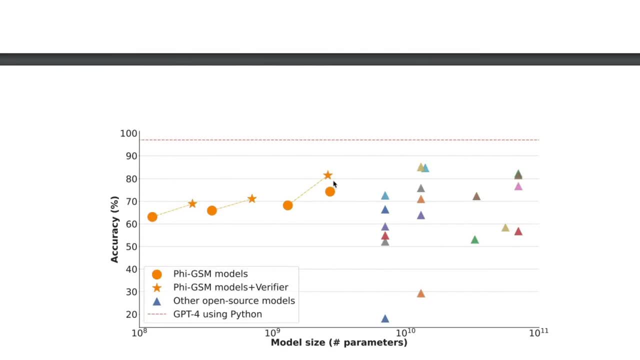 they are going to achieve 81.5% accuracy. I mean, just see, they're going to achieve 81.5% accuracy, while you can see the top line GPT-4 using Python itself is this. So what they're saying is that this 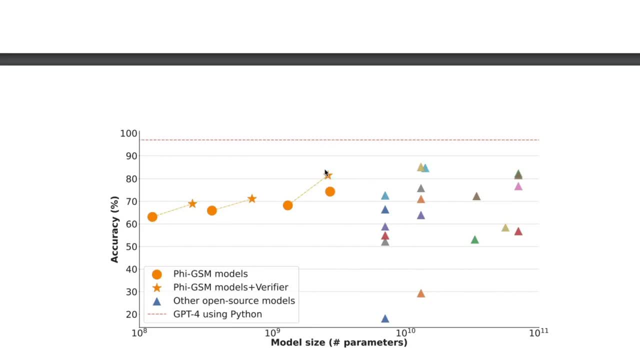 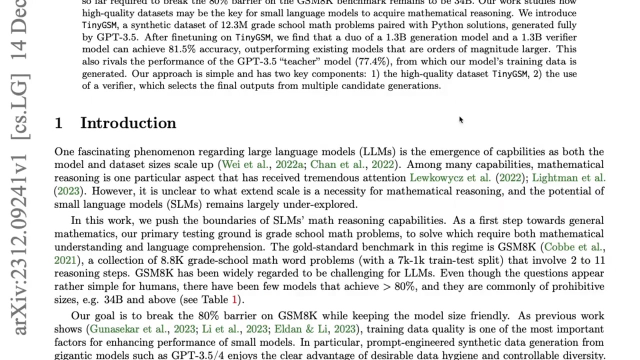 is the gap between a 1.5 million dollars, I was going to say million dollars, 1.5 million parameter model, coupled with a 1.5 million verifier model, and GPT-4 with Python. I honestly want to believe this. I honestly have good faith that this might be a really good model, but I don't know. So the immediate next thing that I did is I was searching for if there is anything related to contamination. 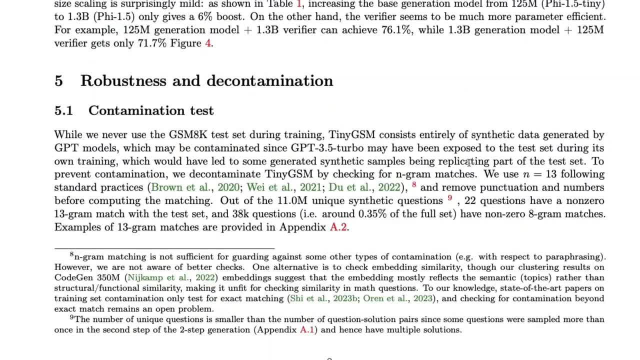 So I was like, okay, fine. The numbers look absurd or numbers look amazing, which is kind of absurd like mental algorithm. So I wanted to see if there is anything contamination. So rightfully, 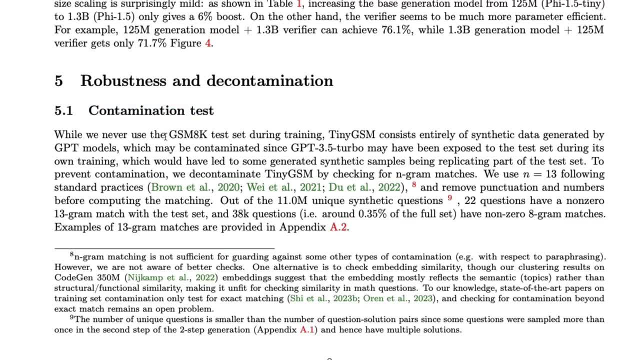 they have a section called contamination text. While we never use the GSM 8K test set during training, which I highly appreciate, when you build a model, you are absolutely not supposed to train the model using the test set of a benchmark. Please do not ever do that. Tiny GSM consists entirely of synthetic data generated by GPT models. Okay. 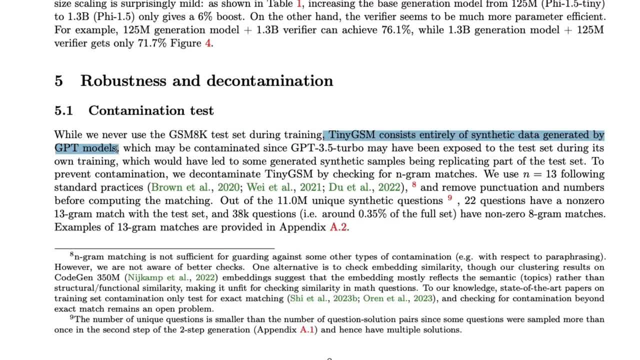 So the way things work is you go to GPT 3.5 turbo, and you send a prompt, you get the response, and you tell the model to also give you a Python code. So this way, you will have the prompt, 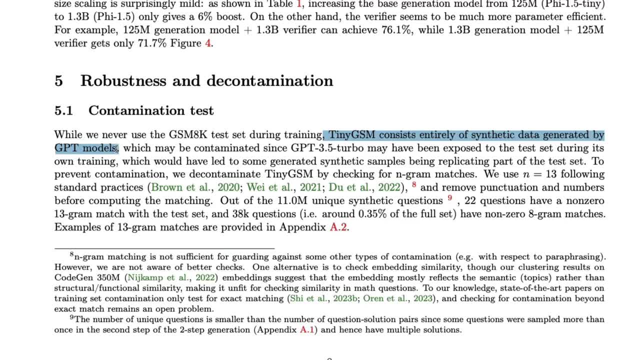 you will have the math problem in itself, and you will have the math solution. So this is how synthetic data is generated, which may be contaminated since GPT 3.5 turbo may have been exposed to the training set, sorry, test set during its own training, which would have led to some synthetic samples. 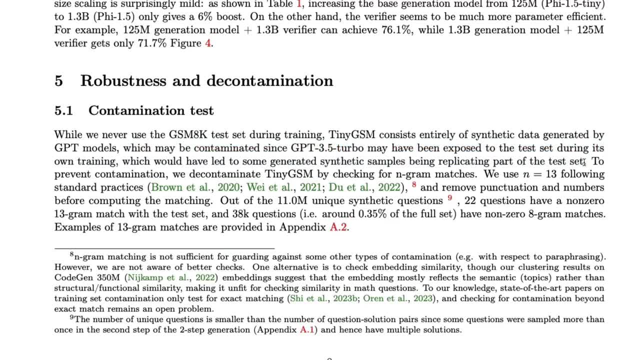 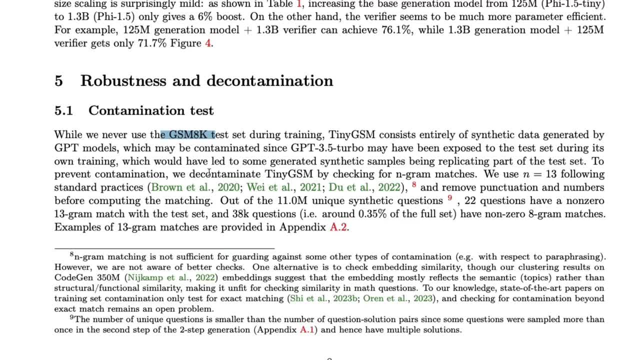 Okay. this so they wanted to prevent contamination like very good researchers do that so we decontaminate tiny gsm by checking for n gram matches my first problem starts with here if you want to decontaminate something i know i know this this is also an established you know technique like for you to decontaminate but if you are going to use only n grams and in this case they are using n is equal to 30 to actually figure out whether the text was an exact match or not and the problem first of all starts here like um even though this is a good paper i like they're a teacher student kind of an approach which we'll soon discuss like i'm not completely going to be ranting about this 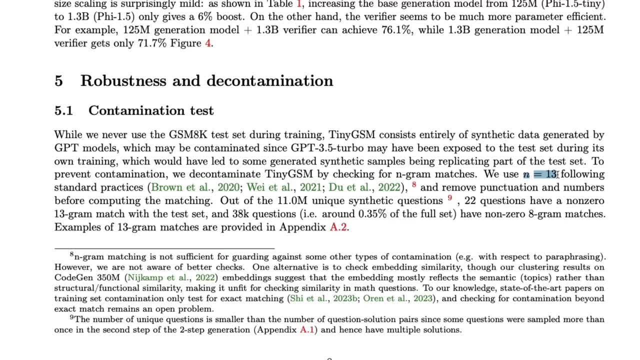 paper even though that's what i'm doing since i started the video so they're using an n equal to 30 n gram so if you are not familiar with n gram so for example if you take this text while we never use their gsm8k one gram would be you split everything into while comma v comma never use v gsm8k by gram or two grams would be while we we never never use use they their gsm8k so like this they are using n is equal to 30 to do the match um they remove the punctuation numbers before computing the matching out of 11 million unique synthetic questions 22 questions have a non-zero 13 gram 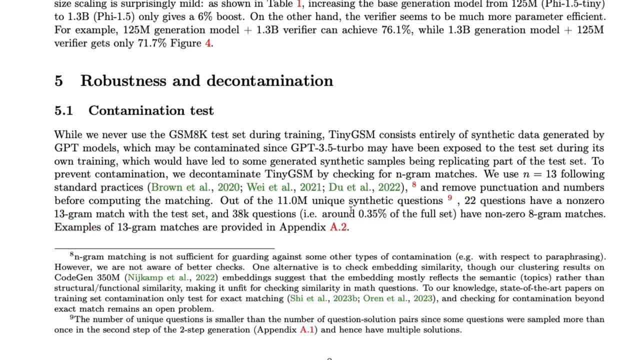 match with the text is so it's a very small percentage like if you see so it's just like 0.35 percent of full set 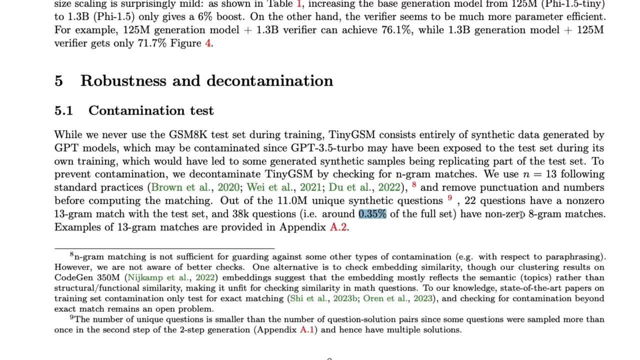 that might make me give them a benefit of doubt but i strongly believe having a 13 gram match is definitely not the right approach which the researchers also agree here one alternative is 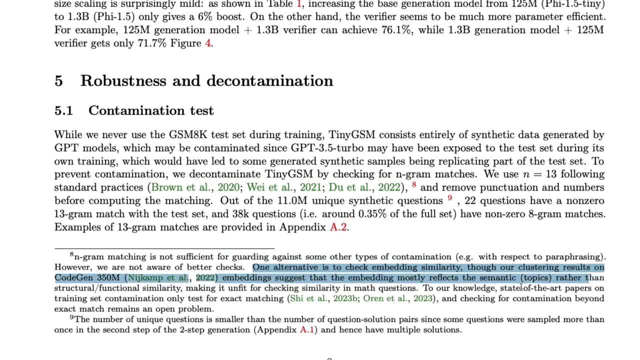 to check the embedding similarity through our clustering results on code gen embedding suggests that the embedding mostly reflects semantic topics rather than the structural functional 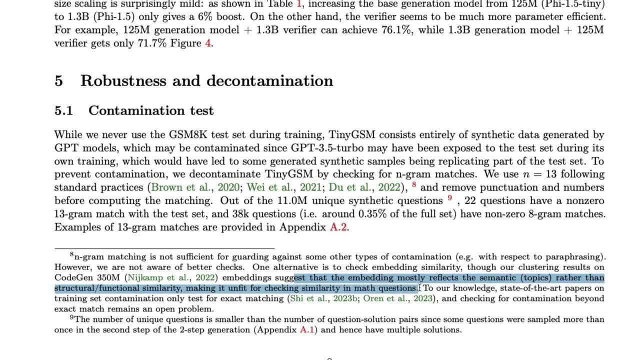 similarity making it unfit for checking some of the questions that we are going to be discussing today so this is a very simple way of checking similarity in the math to our knowledge state of the papers 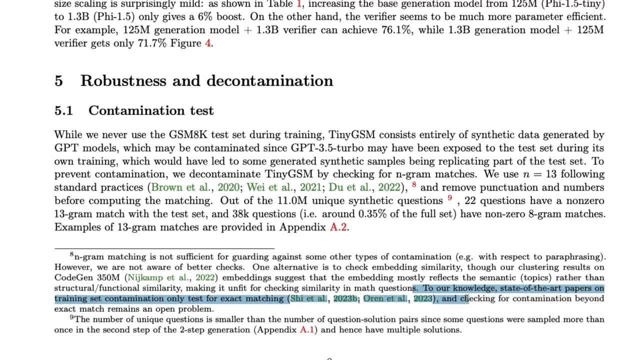 on training set contamination only test for exact matching and checking for contamination beyond exact matching remains an open problem i know this is an open problem but i strongly have my 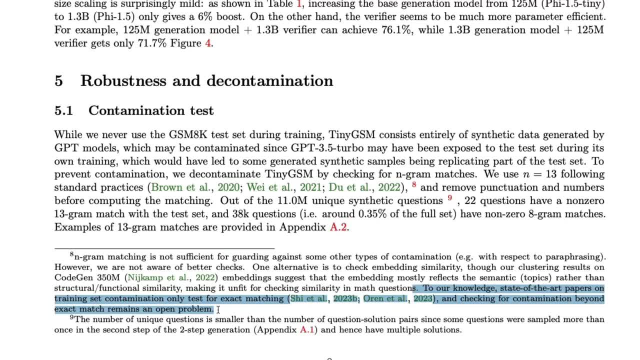 own reservations when you use a large language model like gpt 3.5 turbo to generate a text that might have had knowledge about the benchmark on which you're going to test this i have reservations 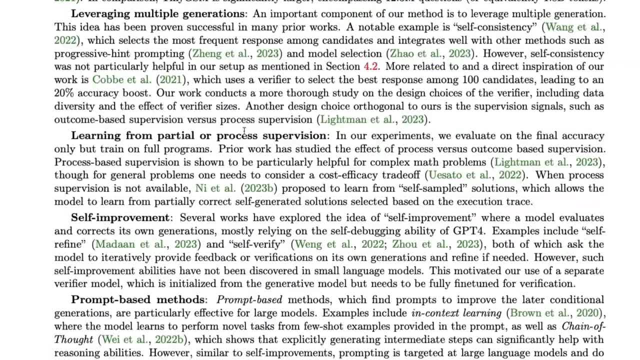 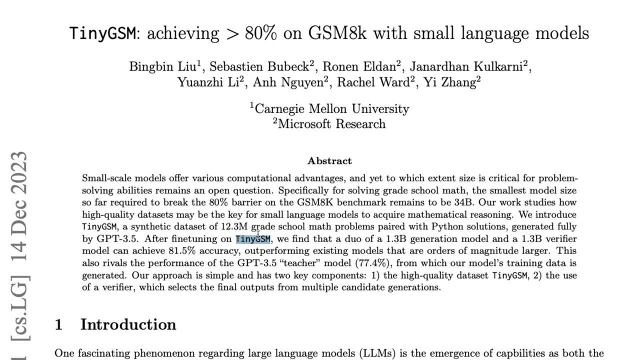 actually get into how good this model is like i want to really appreciate this model so what is this model doing this model is doing two main things like i said like one it is introducing the dataset tiny gsm second it is introducing a teacher student kind of a model so it it up 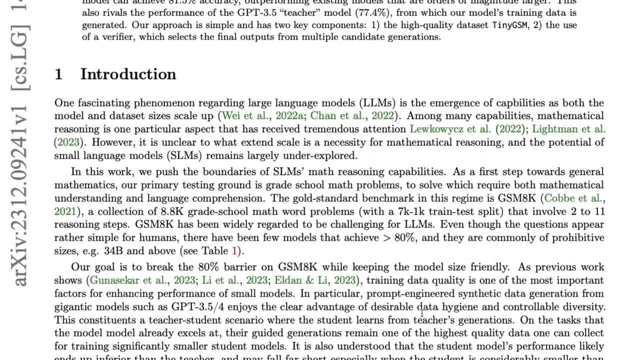 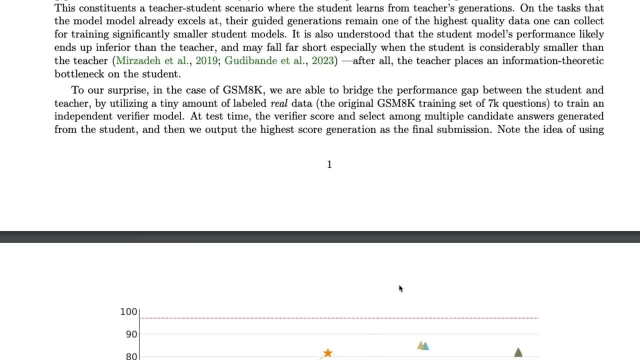 it gives you a text generation model and it gives you a verifier model and that verifier model actually increases the efficacy of whatever this is being generated so first tiny gsm is a 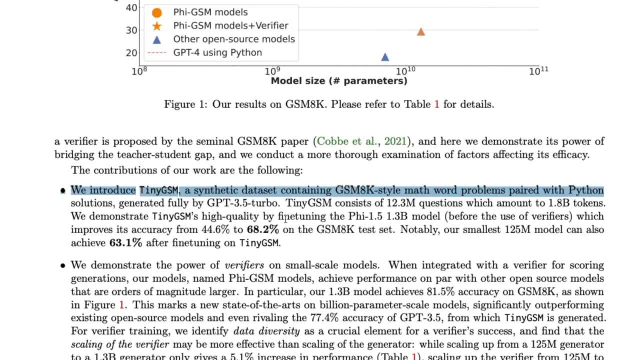 synthetic dataset and when they train or fine-tuned phi 1.5 1.3 billion parameter model not the phi 2 just remember not the phi 2 when before they used verifiers the tiny gsm fine-tuned phi model accuracy improved from 44 to 68 which technically tells me that something is going on but anyway 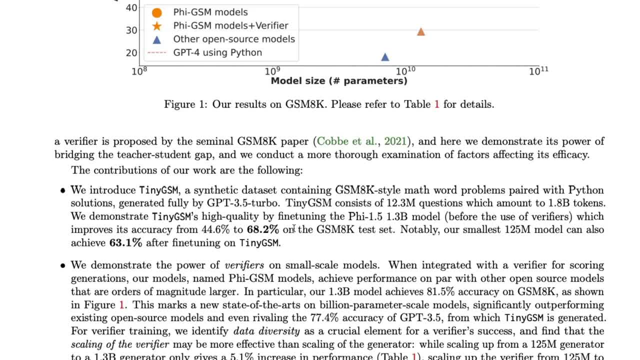 like as i said i have the benefit of doubt i want to appreciate the effort so notably our smallest 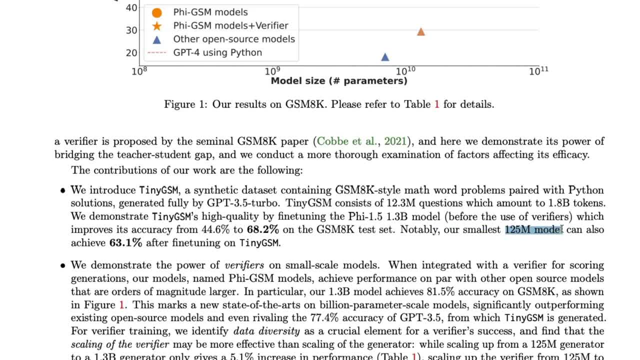 model 125 million parameter model can also achieve 63.1 so what you want me to believe is this is gbt 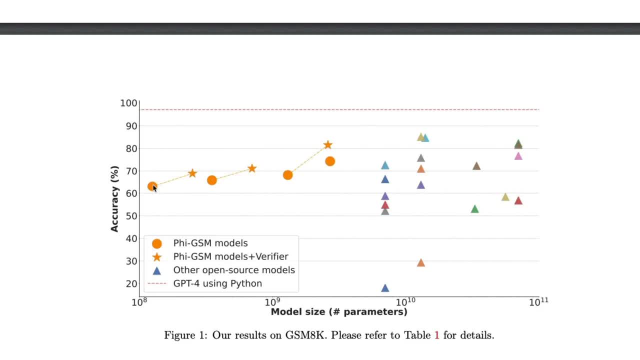 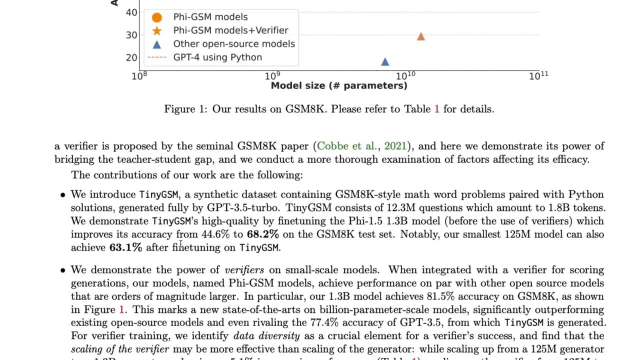 4 this is 125 million parameter and this is the difference i know the difference is like 40 percent maybe like a huge number but i just want to leave you there that is a difference now the next thing is they are actually 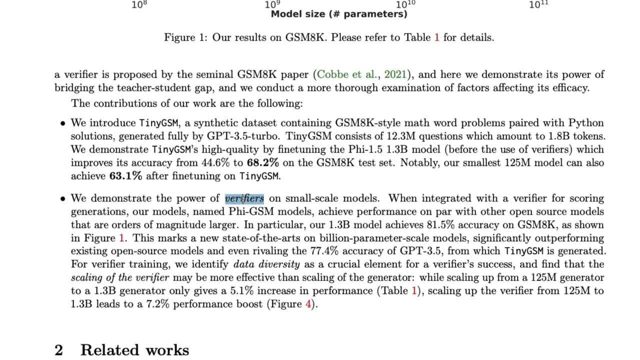 demonstrating that verifiers as a concept can be a huge improvement for the small scale or slms what microsoft loves calling it slms so rather than taking every single output from the large language model that it generates you use a verifier model that would hand pick what the best output would be and then it gives you so this is like reversing of rlhf like typically what you do in rlhf but 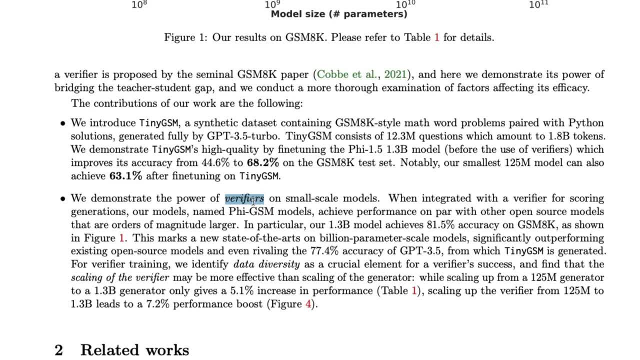 instead of that you have this model that would pick the right approach right uh, output and then you get the output and then that will do and they have said that while scaling up 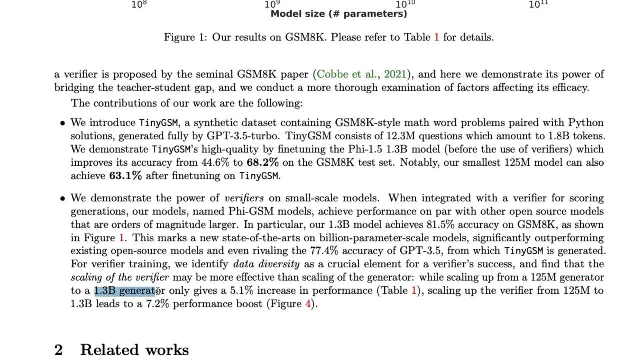 the 125 million generator to a 1.3 million generator so taking a model from 125 million parameters to 1.3 billion so this is like 10 times increase gave only 5 percent increase in 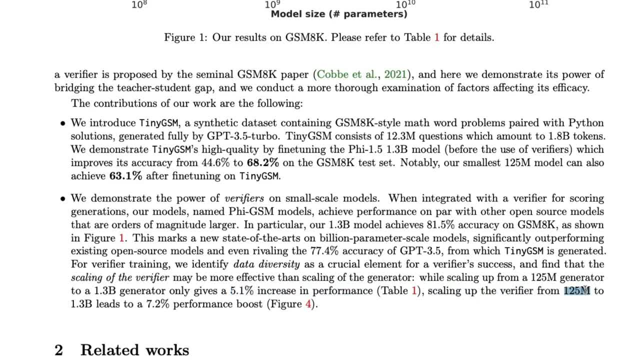 performance while scaling up the verifier from 125 million parameters to 1.3 led to 7 percent so you can see the difference right so the difference one is the generator model second one is a verifier 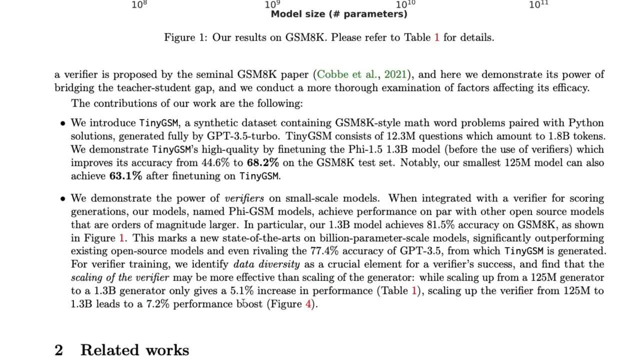 model this seems like a good difference now i'm going to get back into the rant mode the rant 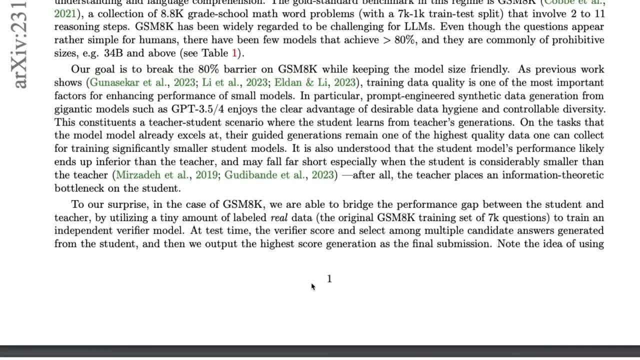 mode is because how is the verifier model built here like even though i love the concept of verifier models i love the concept of teacher model and student model how is the verifier built 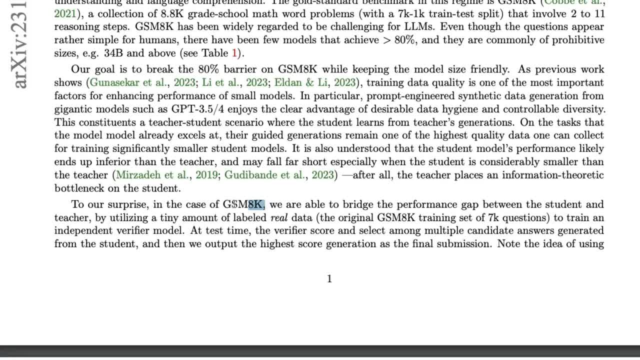 to our surprise in the case of gsm 8k that is a that is a benchmark against which like all these metrics are being measured against we are able to bridge the performance 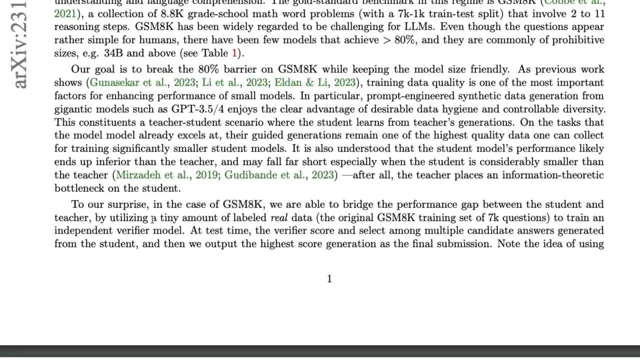 gap between the student and the teacher by utilizing a tiny amount of labeled real data 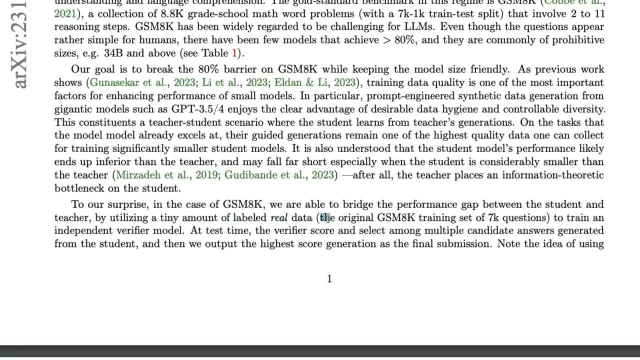 where is it real data coming from the real data is coming from the original gsm 8k training set 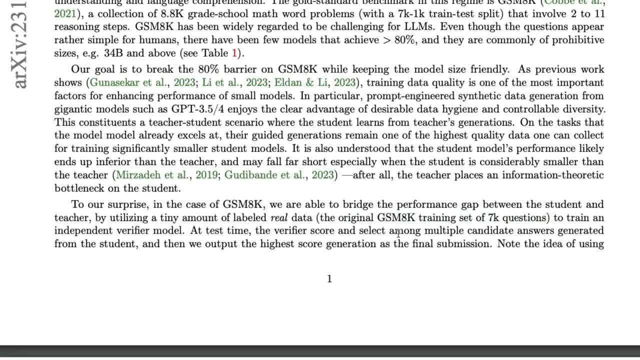 of seven questions sorry seven thousand questions so they took seven thousand questions from gsm 8k 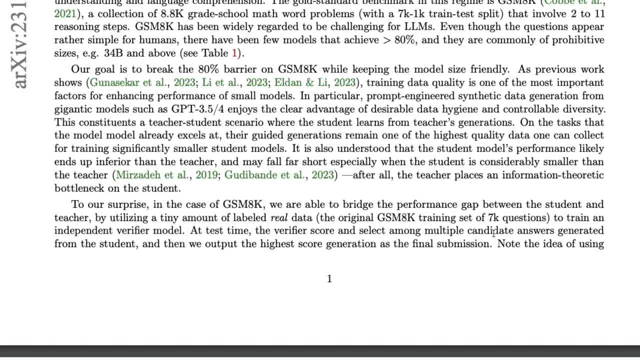 training set now in their difference they can say they did not use the test data which i really 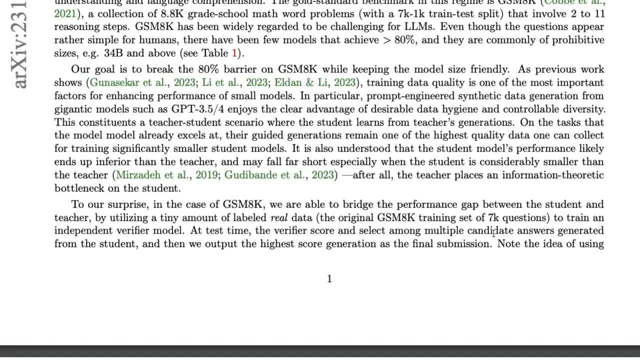 appreciate but they used gsm 8k training set seven thousand questions from this and trained an independent verifier model independent how independent it is okay at test time the 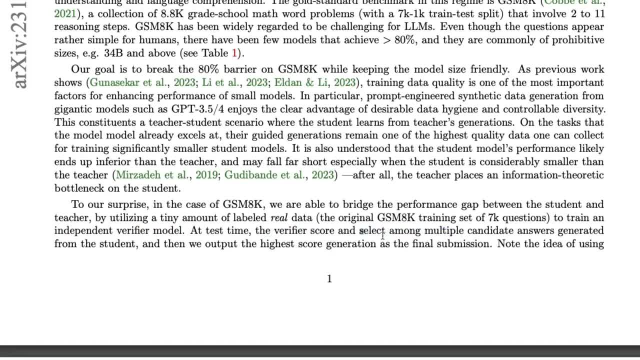 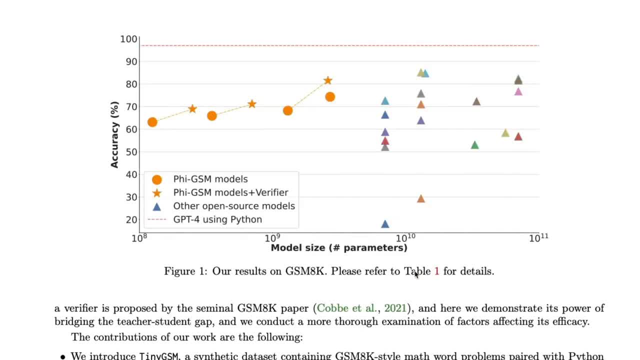 verifier score and score the responses select among multiple candidate answers generated from the student model then we output the highest score generation as the final submission so while this 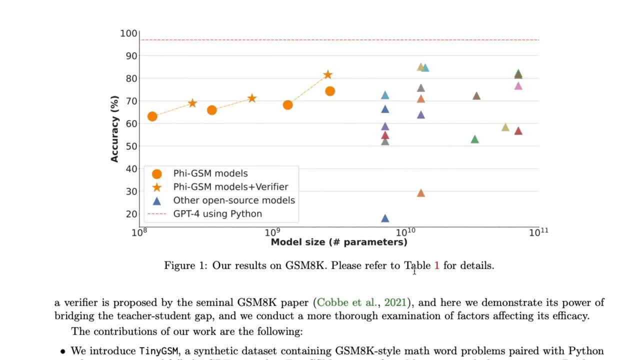 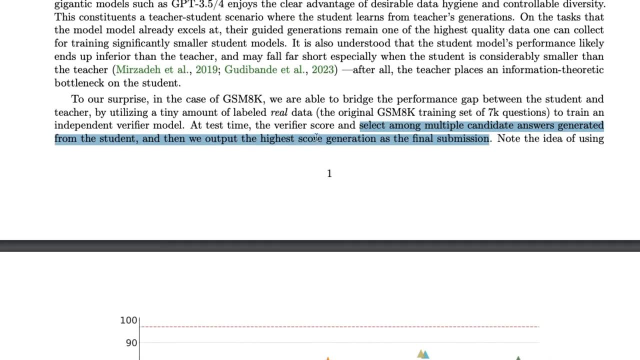 approach is really good like i strongly believe that you need to have this kind of multiple layers to get really good things out of this model once again i have my reservations about how this model 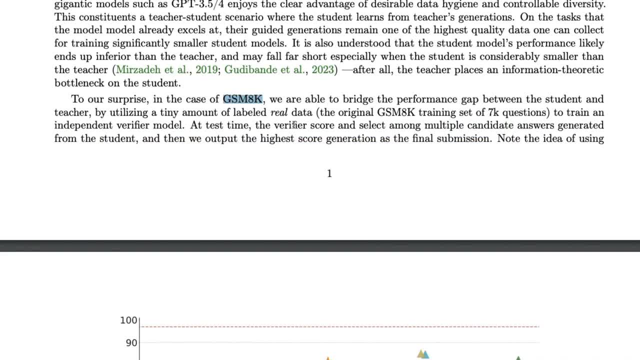 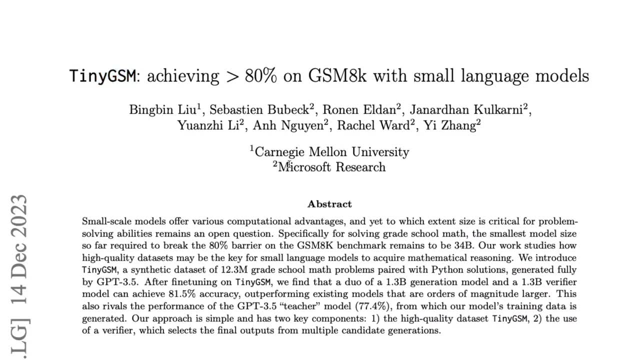 is gonna interact with an intermediate experiment so we will dive into the training learning 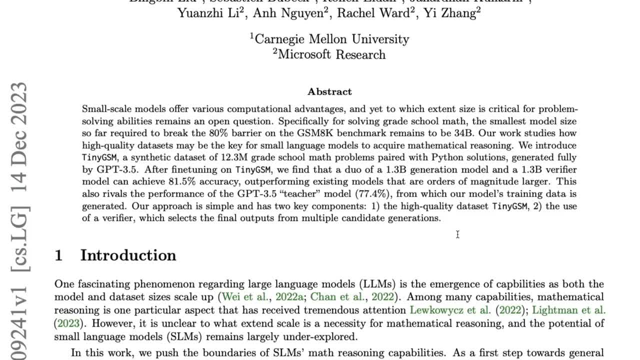 and yap demo in light of the fact that the training model and where we are tests are verg avec mode test event setup it is a very fair model from the benchmark data set while 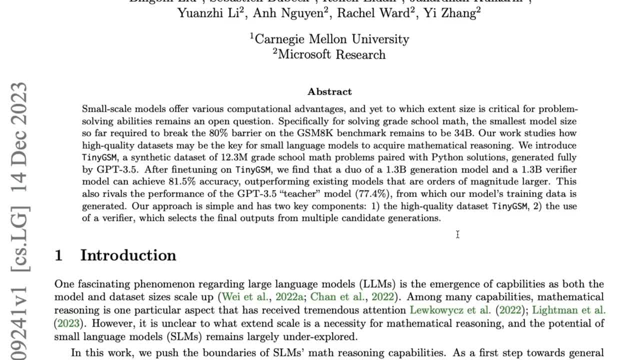 it is even training lead is it so overall i want to stop this video here i appreciate tiny gsm data opened by a few model rather than having a teacher always correcting students answer sheets you can have 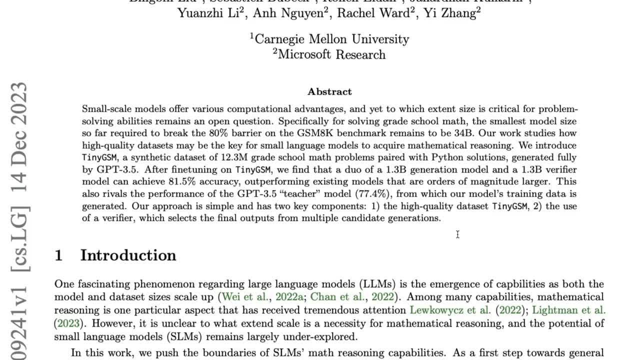 this kind of model validating teaches i think these kind of models would be really good at these kind of tasks which i do not disagree at all but i'm just like generally trying to think 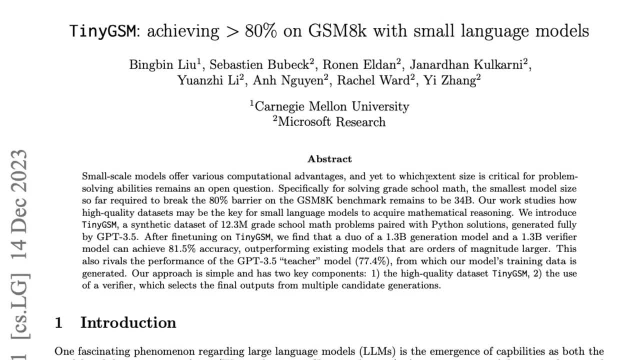 at this point that what is that we are trying to do if we want to advance large language models are we trying to build more and more models just to hit the leaderboard um are we trying to innovate 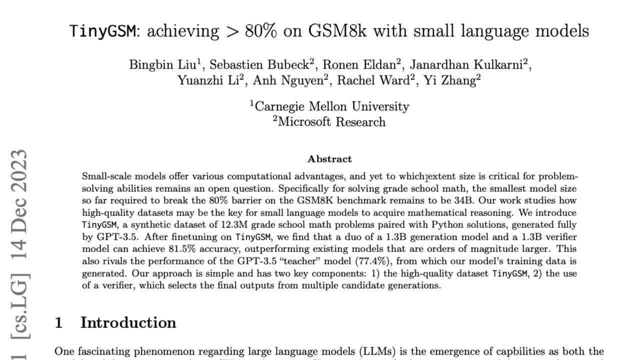 new solutions approaches new methodologies i i don't know like i think i'm i'm losing track of what is happening in this space while i'm very happy with the smaller models while i'm very 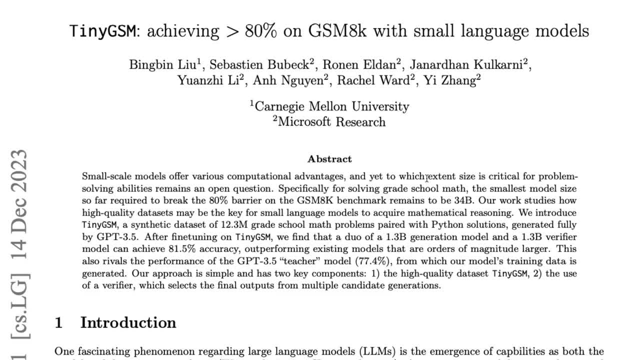 happy with the approaches that they've done i'm not i'm not able to come terms with how they have taken a data set how they have gone like deep into having like a synthetic data set for math and which might have had some kind of gsm 8k data 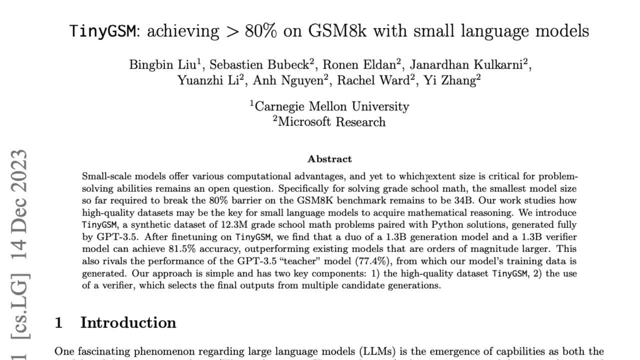 and then they have validated it i would have absolutely loved this much more had they have used a different benchmark 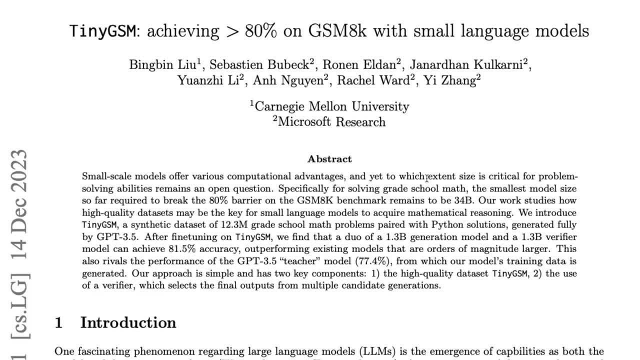 totally something like i think recently one thing that is popping up is like the hungary math result or hungary high school result so you could have used some data set that has not been exposed to this let's say gpt 3.5 gpt 4 and they could have verified it i don't know i feel like something is 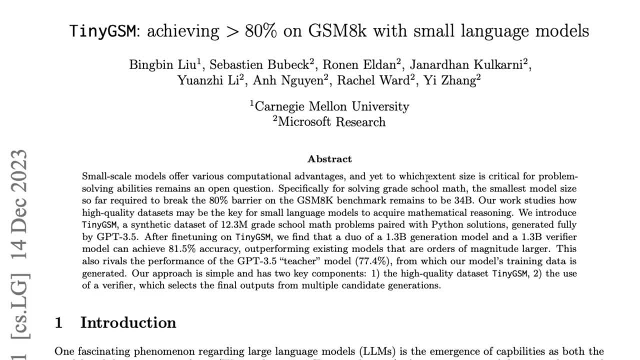 not 100 good about this but i also strongly appreciate the kind of efforts that have gone 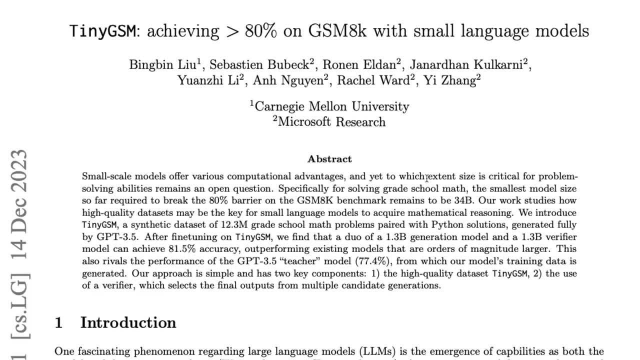 into this in building a small small small a large model or small scale large model that can probably have its own computational advantages